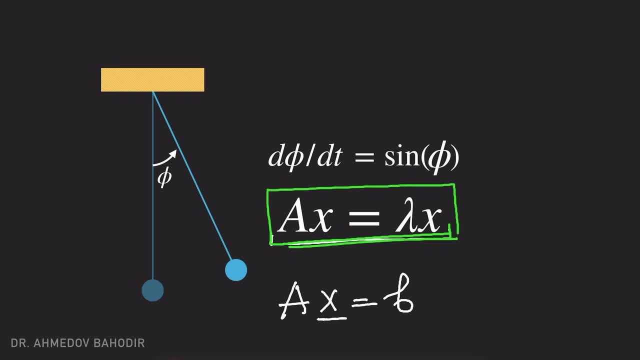 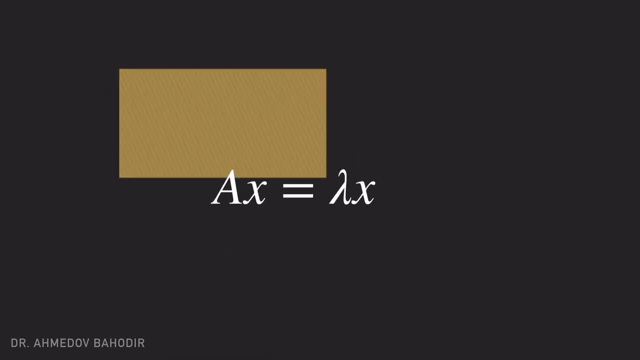 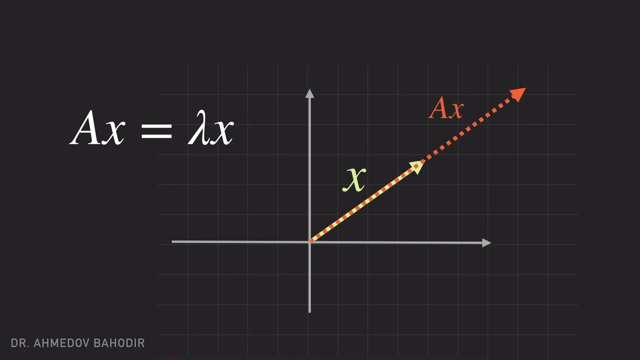 this type of the problems is called the Gauss-Jordan elimination method. So let's look at this equation in more detail. So let's say x is given some vector and A-axis is going to be another vector which is going to be parallel to the same vector. 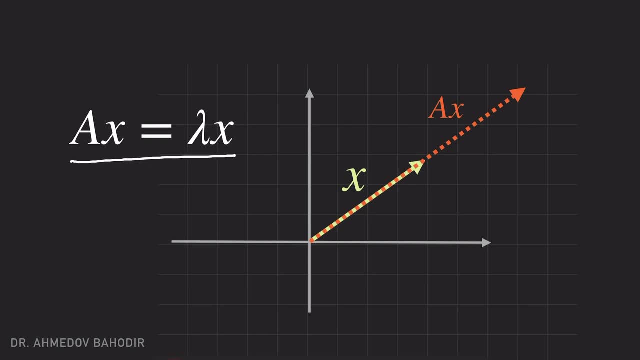 So this is, what does it mean, this equation? You see, so if you multiply the vector x to the A, to the matrix A, you get the following equation: It's going to be again a vector, And you see so. do you remember? previously we said that hey, if you are given two vectors, 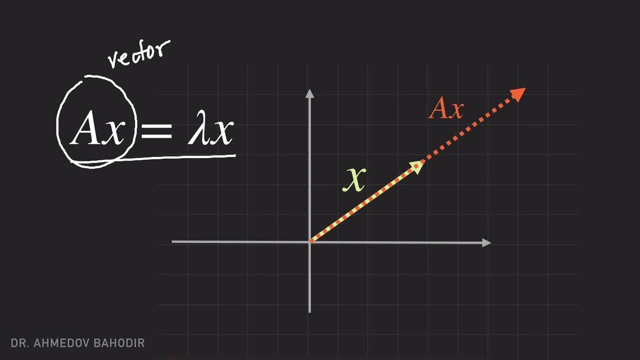 which are parallel. then you can obtain the second vector, so this red vector, by just multiplying the yellow vector to some constant. So this is going to be our red vector, right? So essentially they are the parallel vectors, and that's what this equation is going to. 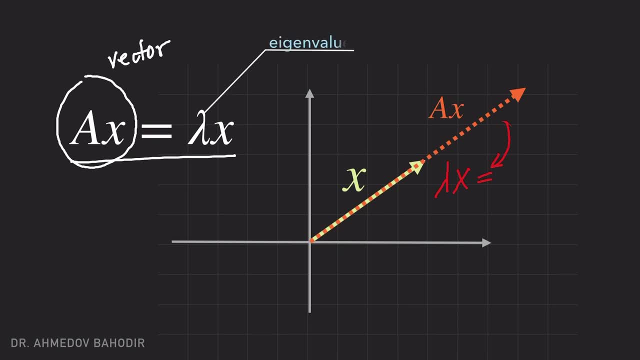 tell us. So if you multiply the vector x to some vector, to some matrix A, it is going to give you some vector which is parallel to the x itself. Okay, So this vector A times x is going to be parallel to this x. 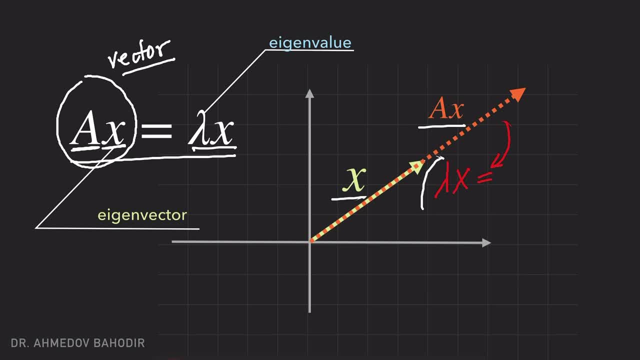 And essentially this constant which basically is going to scale this vector x in order to get the same vector as A. x is going to be called as an eigenvalue And this kind of vectors which are basically specific for different types of the matrices. 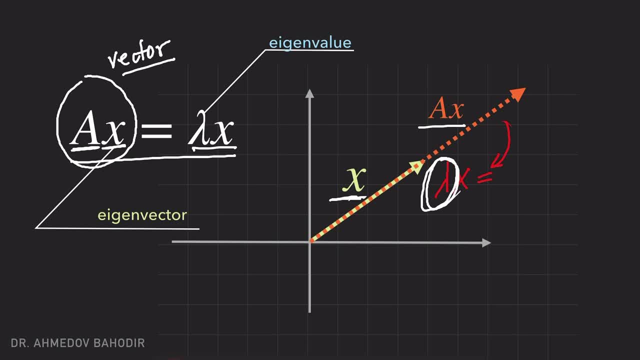 are going to be called as the eigenvectors. So the word eigenvalue is coming from the German word eigenwert, which basically means its own value. So essentially the own values of the matrices And we will see later on in its applications. so their meaning is essentially the important. 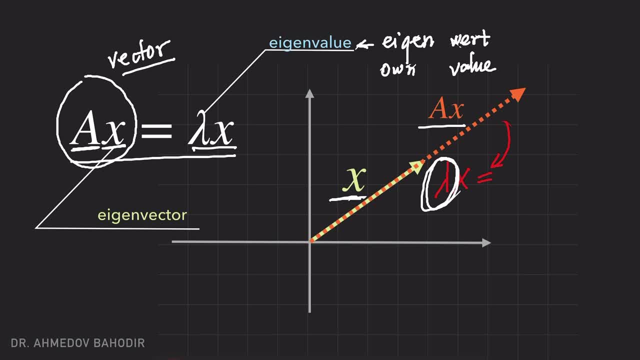 values. They are going to tell us the most important values of the matrices. So let's discuss again a bit about the eigenvalue problem. So again, the eigenvalues or eigenvectors, is such a vector x so that when you multiply 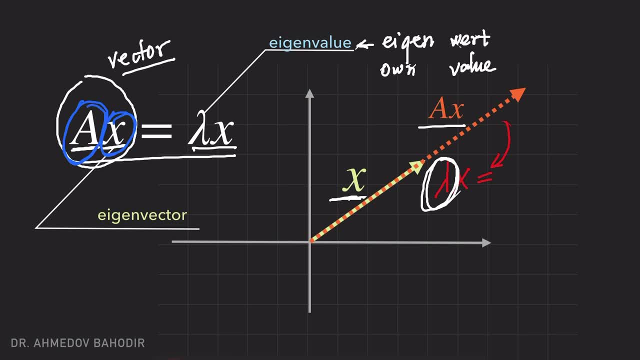 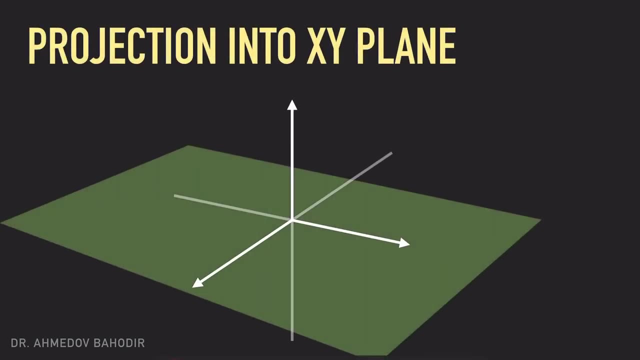 these vectors to the A, You are going to get a vector which is going to be parallel to this vector itself. So let's consider some examples. So let's say we are given the projection matrices. So previously we talked about the projection matrices. 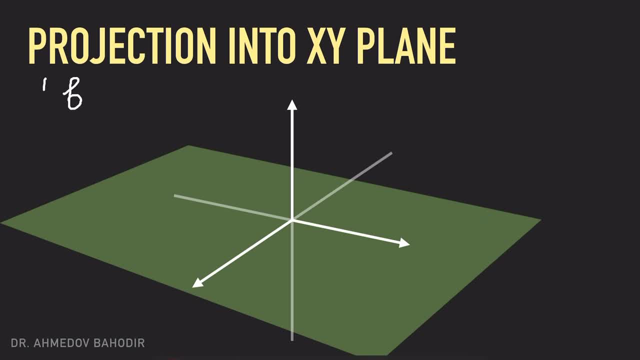 So we say that, hey, if you're given any vector b and if you multiply this to some projection matrix p, it's going to project this vector p onto the subspace, Right? So let's say we are given the xy plane and we would like to project or find a projection. 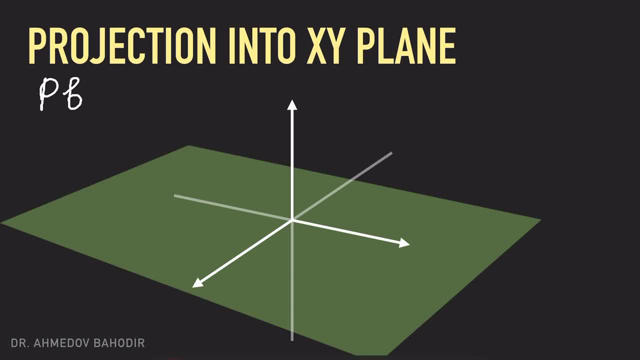 of any vector onto this plane. So, essentially, if you're given some vector b, by just multiplying this vector b to this projection matrix p, we can obtain this yellow vector which is going to be on this plane. Well, the only question is: could you figure out the vector b? 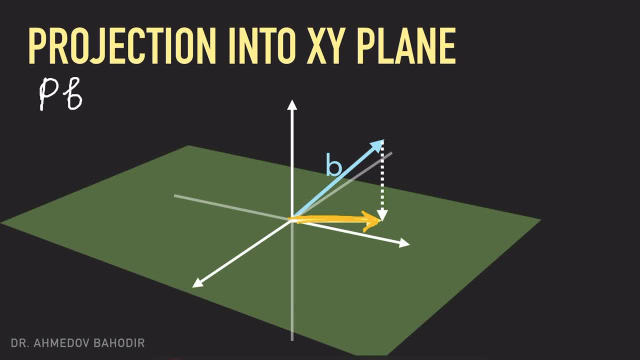 Such a vector b, so it might be any vector b, so that the projection of this vector b is going to be parallel to this vector b itself. So let me write this: So what is the b? what's a b vector, so that its projection is parallel to itself? 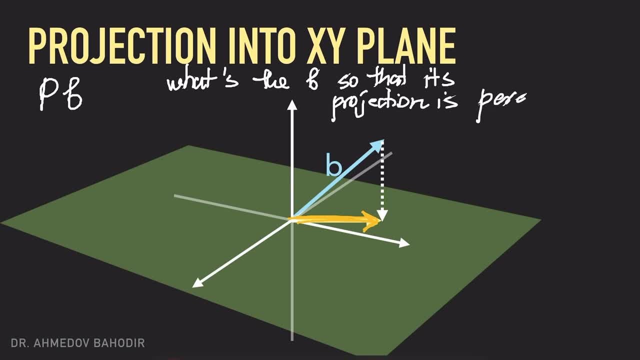 Okay, So it's a vector. Okay, Okay, So it's going to be parallel to itself. So far, from this picture, it is clear that the yellow vector is not parallel to the blue vector. Well, if I would like to find such a vector b whose projection is going to be parallel. 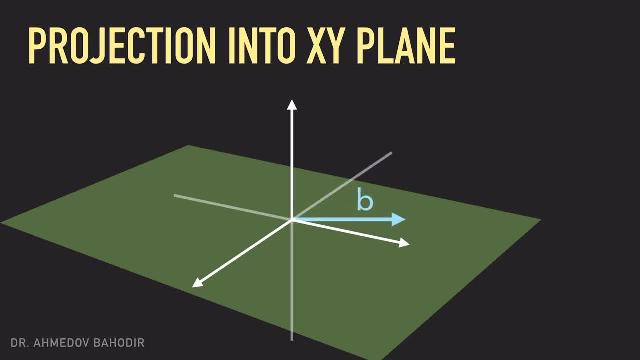 to itself. I probably need to choose this vector b from the plane. Well, the projection of this vector b onto the subspace- Okay, Onto this plane, is going to be the same vector b. So let's say p matrix is going to project, project any vector onto this plane. xy plane. 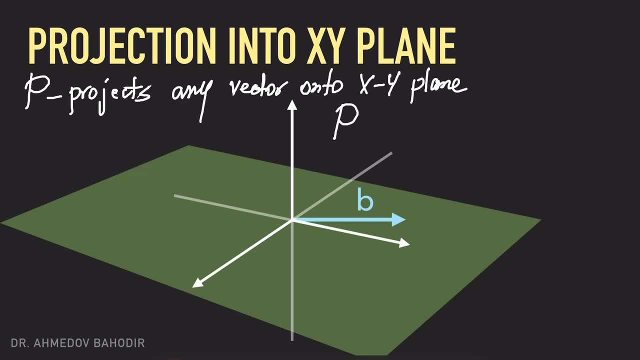 And in this case, the projection of this vector b onto this xy plane is going to be itself right. So what is the eigenvalue in this case? So the eigenvalue in this case is going to be equal to the 1. And the eigenvalue, the eigenvector, sorry- is going to be any vector on this plane. 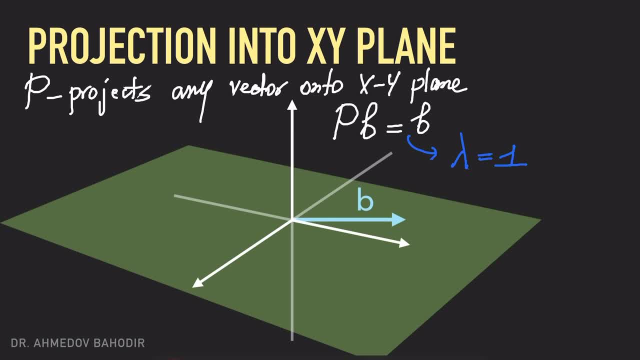 Well, so we are going to have another vector. So here, another eigenvector. So can you just think about this problem a little bit in more detail, so you can pause this video and think about this in more details And figure out the vector b so that its projection is going to be parallel to itself? 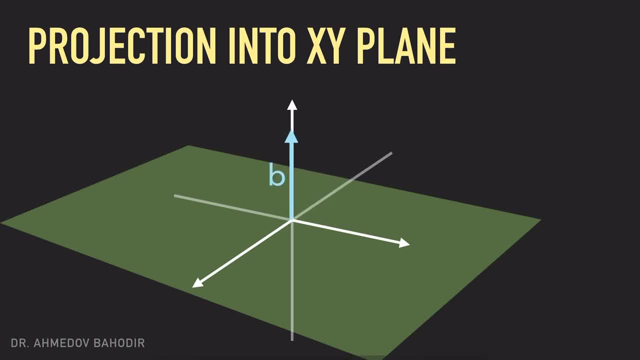 Well, probably I need to choose the vector b along the z-axis, Then the projection of this vector b onto the xy plane would be simply this point, or this vector zero, vector Right And again. so, if you are given the matrix p, which projects this point, 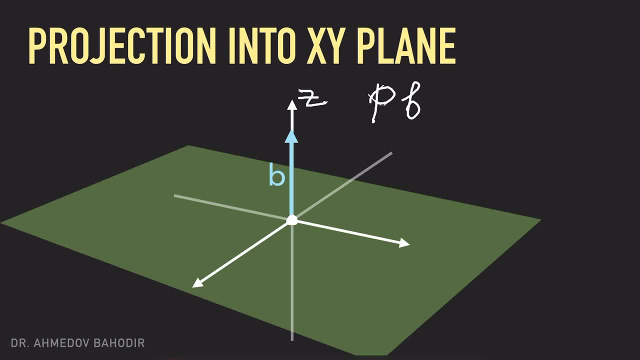 Any vector b onto the xy plane. And if you are given a vector along the z-axis, its projection onto the xy plane is going to be simply zero vector. And in this case, what's going to be the eigenvalue? The eigenvalue in this case- so let me denote this as a lambda 2, is going to be simply: 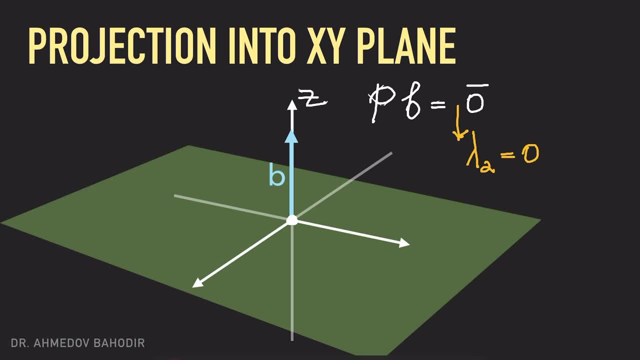 equal to the zero right. So this is the factor which makes which essentially zero vector. Zero vector is parallel to any vector right And we can obtain this by just scaling any vector, by multiplying any vector to the zero. 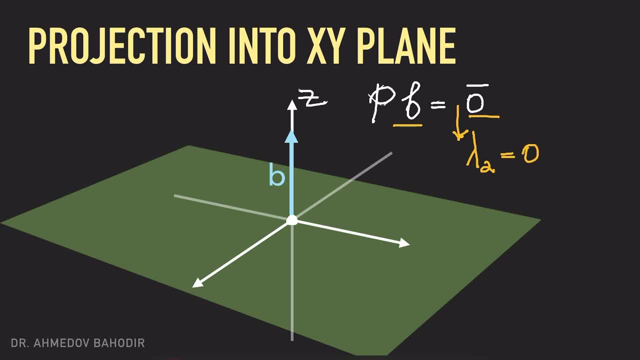 right. So this vector and this vector are equal, and the scaling constant is equal to the zero, which is the eigenvalue. You see, so for this matrix, which projects any vector onto the xy plane, we've got two eigenvalues. 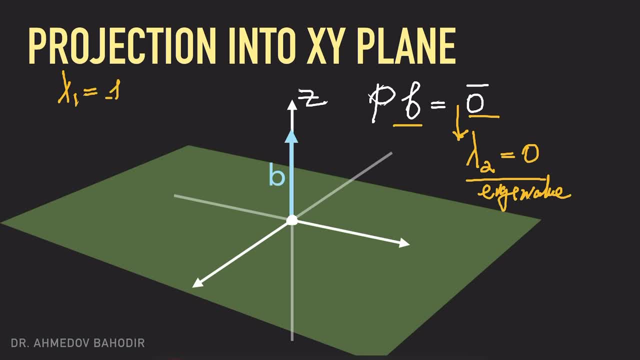 The first eigenvalue used to be equal to the one and our eigenvector is going to be any vector on on this plane, xy plane- And we found the second eigenvalue. so the second eigenvalue is equal to zero And this vector eigenvector is going to be on the z-axis. 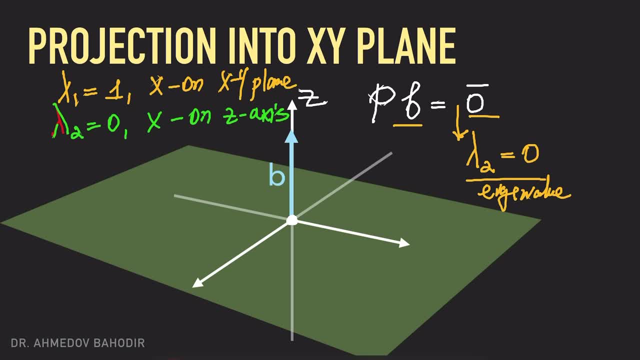 So we would like to try to reveal a couple of more problems, A couple of more properties about eigenvalues and eigenvectors, so that you will try to understand this a little bit in more detail, a little bit more deeply. So let's consider another example. 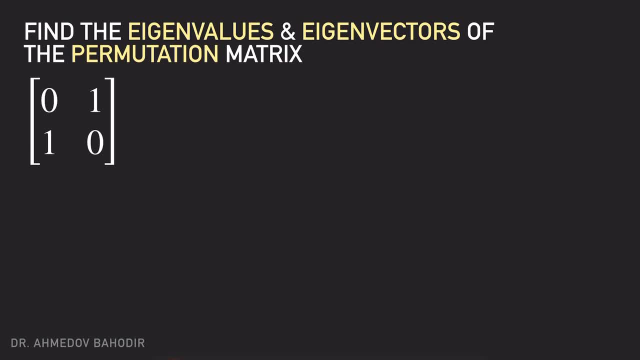 So let's say we are given the permutation matrix and we would like to figure out its eigenvalues and eigenvectors. So what does this permutation matrix is actually? If you multiply this p-permutation matrix into some vector with the two rows, it's going: 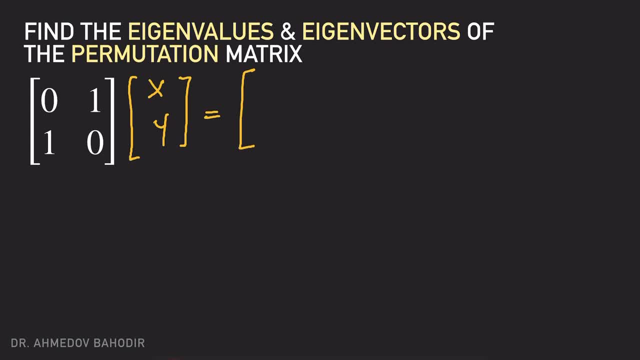 to simply interchange the rows. it's going to be right. say y and x. Now could you please figure out a vector so that if you interchange its rows it's still going to be parallel to itself? Well, maybe it's going to be the same right. 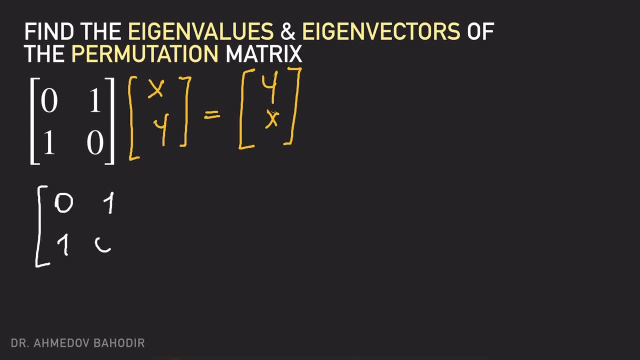 So, for example, it's going to be zero, one one, zero. So what is this vector? so that if you interchange the rows it's going to be the same vector as itself? Okay, So hopefully it's going to be one and one, right. 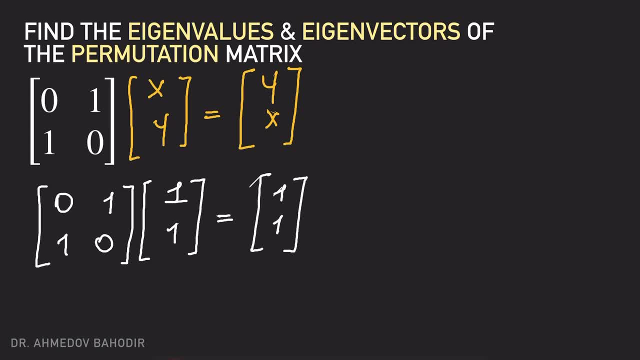 And this is equal to zero. one and one again. So you see. so it brought to you this problem. So the p times the vector x is simply equal to the x, right? What's the eigenvalue in this case? Say the eigenvalue in this case. so let me denote this with a different color: eigenvalue. 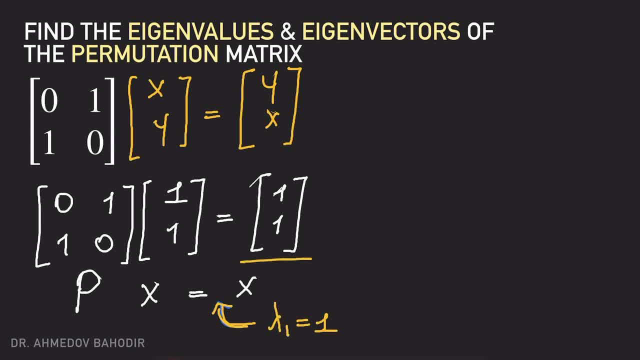 in this case, is going to be simply equal to the one And the eigenvector. is this vector one and one? Now think about this problem a little bit in more detail. So since this matrix is two by two matrix, it probably has a second eigenvalue as well. 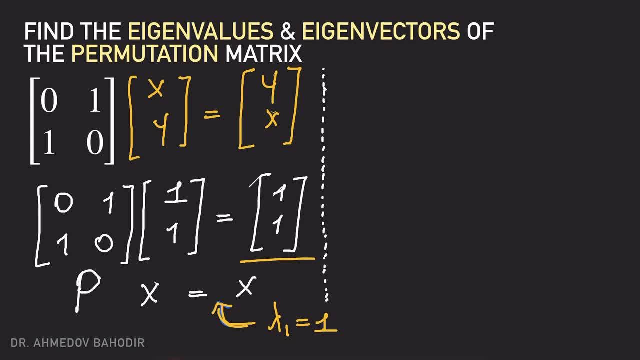 And what might be the second eigenvalue in this case? So probably, if I would choose zero, one, one and zero and the eigenvector as the vector minus one and one, then by just multiplying this permutation matrix to this vector I. 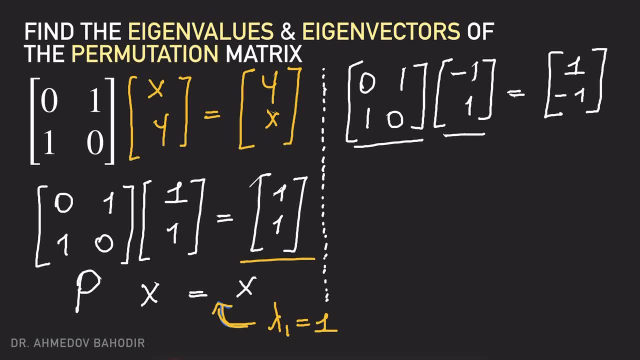 would obtain the vector by interchanging the rows, right. But you know, this vector is parallel to itself, So it's going to be one and one. It's going to be equal to this vector. We can even draw these vectors, right.